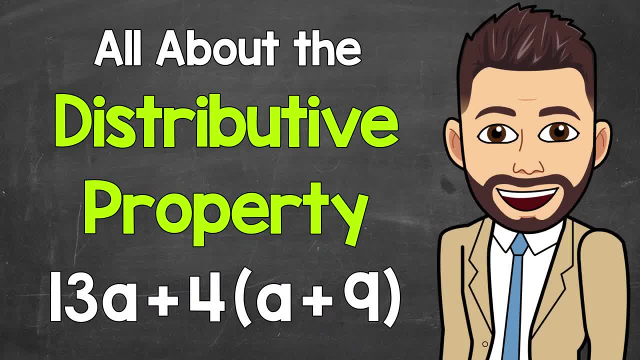 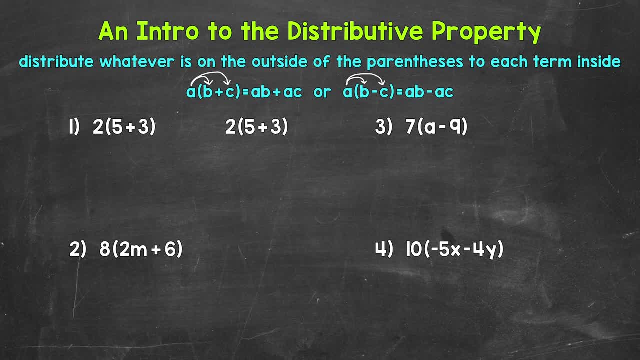 Welcome to Math with Mr J. In this video I'm going to cover the distributive property and how we can use the distributive property to simplify algebraic expressions. We will start with an introduction, After that we will take a look at more examples and then, lastly, we will look at some algebraic expressions. 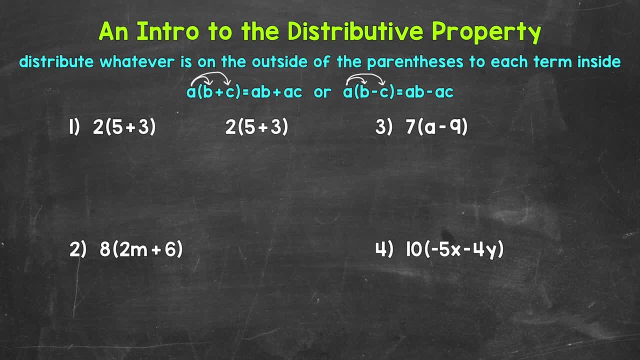 that we will need to simplify using the distributive property and combining like terms. Now, the distributive property can help us remove parentheses within algebraic expressions. This helps us simplify expressions when we do not have like terms within parentheses that we can combine. Now remember, when we have something next to parentheses, that means multiplication. 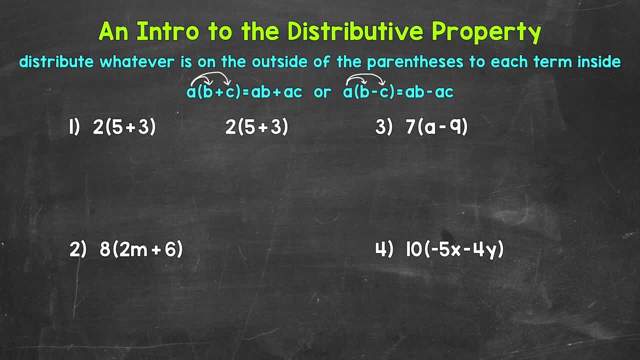 So we can use the distributive property to distribute whatever is on the outside of the parentheses to the terms inside the parentheses. The distributive property works when we have addition or subtraction inside of the parentheses. So at the top of the screen there is a general overview of the distributive property. where A is being distributed to the 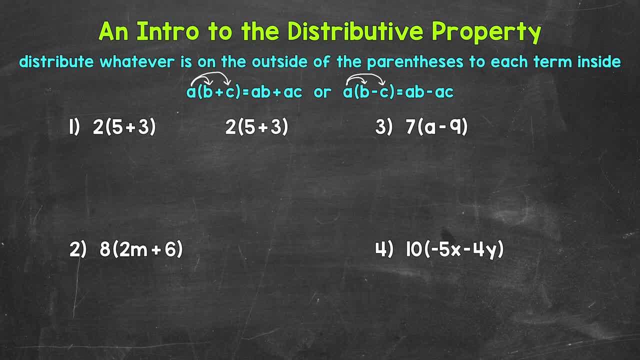 terms inside of the parentheses, The distributive property, and that overview will make a lot more sense as we go through our examples. Let's jump into number one, where we have 2 and then, in parentheses, 5 plus 3. And we're going to do this two different ways. 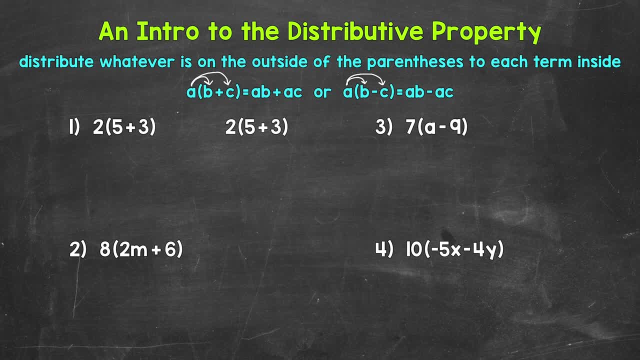 ways by using the order of operations, So doing what's in the parentheses first and then also using the distributive property. Now for number one. we don't have any variables involved. We are actually able to add what's in the parentheses first and then go from there. We don't have to. 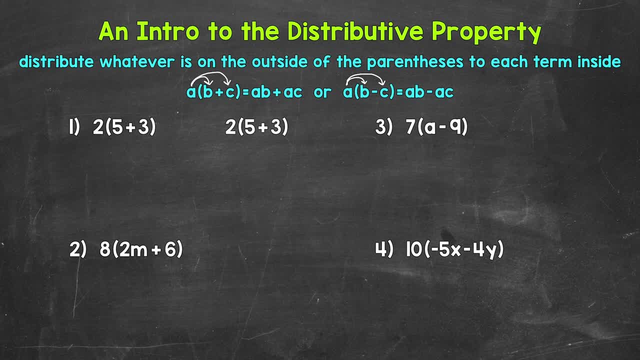 use the distributive property. But the point of number one is to show us that we get the same thing either way. This is going to show us that the distributive property doesn't change the value of an expression. we are able to use this strategy, So again, we get the same thing either. 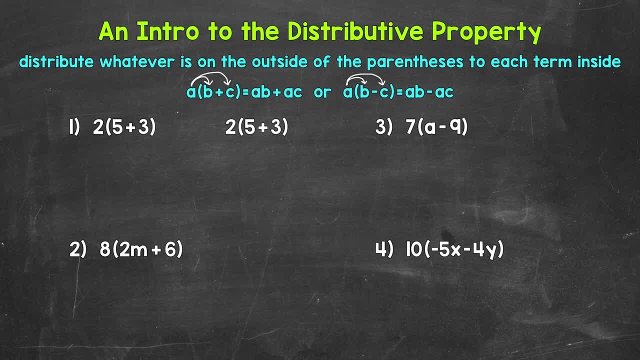 way. Let's start by using the order of operations and doing what's in the parentheses. First we have five plus three, which is eight. bring down the two, And now we have two times eight, which is 16.. Now let's use the distributive property and see if we still get 16.. So we 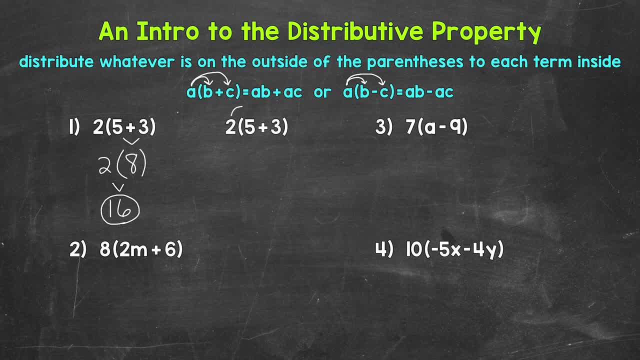 need to take that two on the outside of the parentheses and distribute it to the five and to the three. So we have two times five plus two times three. Two times five gives us 10, plus two times three gives us six. 10 plus six is 16.. 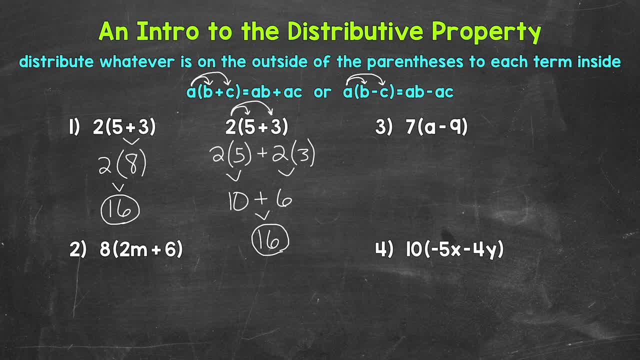 So we get 16 that way as well. So we can see that the distributive property doesn't change the value of an expression and we are able to use it. Let's move on to number two, where we will apply this to an algebraic expression. in order to simplify the expression, we are going to remove the 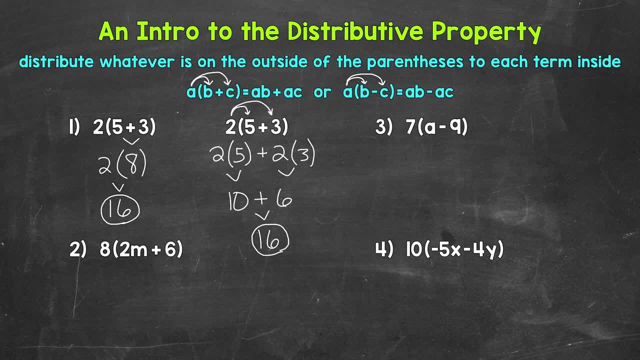 parentheses For number two we have eight and then in parentheses two m plus six. Now we can't combine those terms in the parentheses. So what we can do is we can use the algebraic expression and do, we can use the distributive property to remove those parentheses and simplify this. 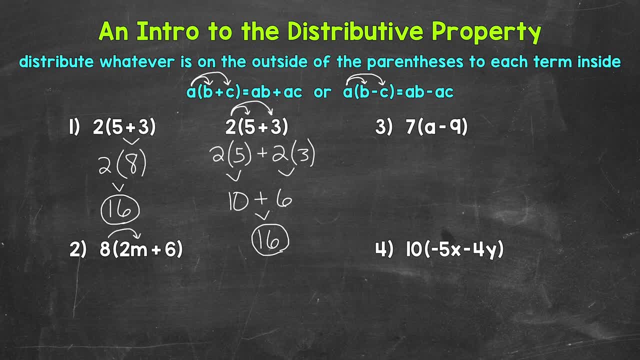 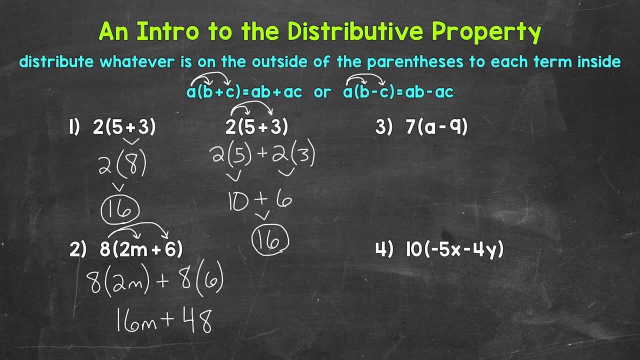 expression. So let's distribute the eight to the two m and to the six. This gives us eight times two m plus eight times six. Eight times two m is 16 m, plus eight times six is 48.. Now 16 m and 48 are unlike terms, So we don't have any terms that we can combine. 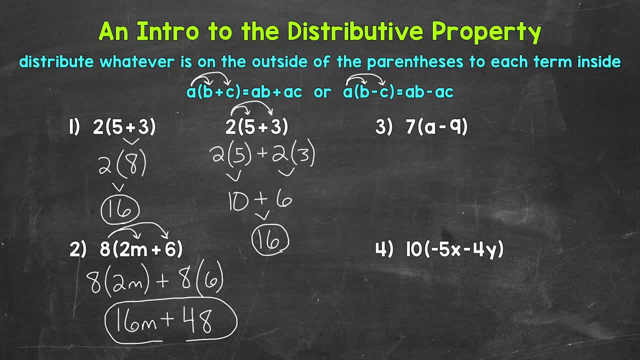 So we are done here. 16 m plus 48 is our simplified expression. Let's move on to number three, where we have seven and then, in parentheses, a minus nine. Let's distribute that seven to the a and to the nine. That gives us seven times a minus. bring the subtraction, sign down seven. 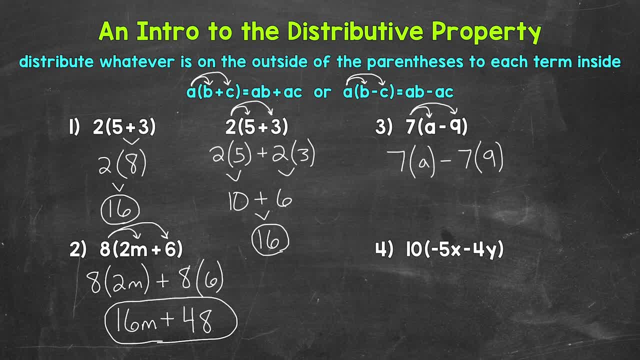 times nine. Seven times a is just seven. a minus seven times nine is 63. So we end up with seven a minus 63. We don't have any like terms that we can combine. So we are done here. Let's move on to number. 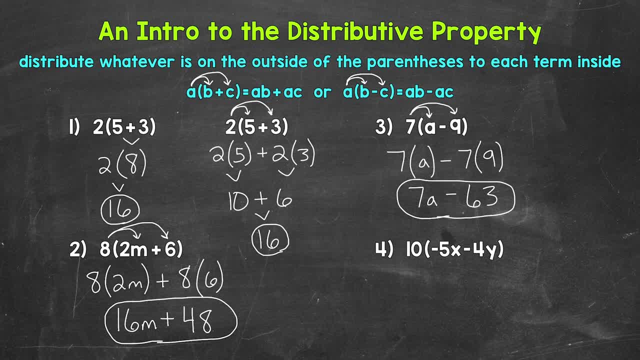 three, where we have seven, and then in parentheses, a plus eight times six is 48. So we don't have any terms that we can combine. So we are simplified and done Again: seven a minus 63. Now I do want to mention another way to think through this. 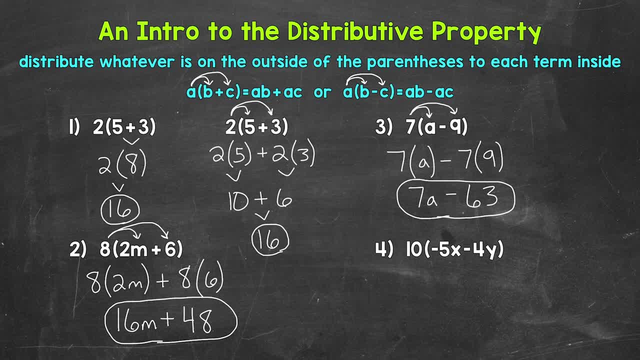 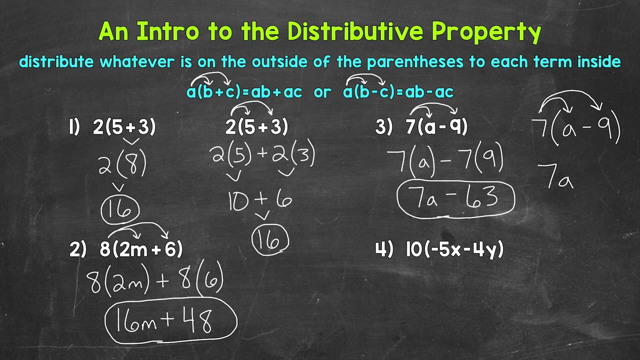 And this is another way to think through whenever subtraction or negatives are involved. So let me rewrite the expression and then distribute the seven, So we have seven times a, which is seven a minus 63. And then we can think of that subtraction sign and the nine as a negative nine, So including. 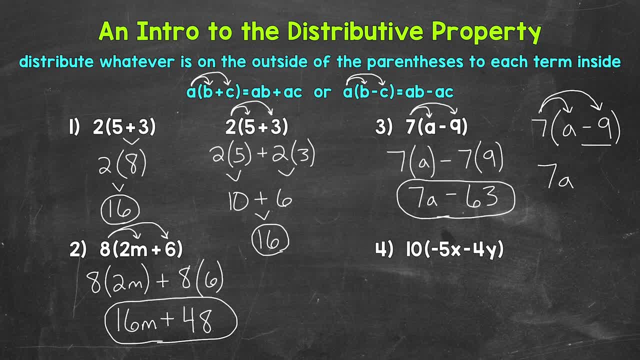 the sign in front with the nine. So we think of that as a negative nine. So let's distribute that seven to the negative nine. Seven times negative nine is negative 63. So negative 63. And we get seven, a minus 63. That way we have a negative nine. So we have a negative nine. So we have a negative nine. 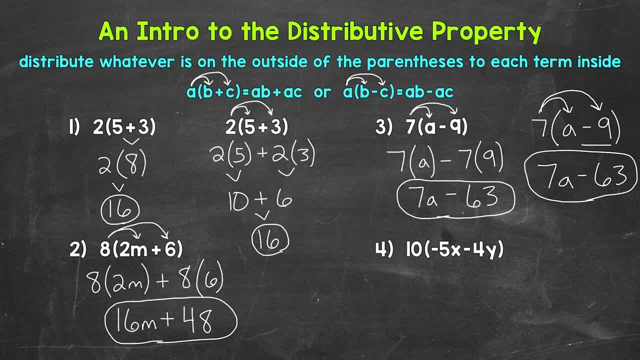 As well, And again, that's just a different way to think through it. You get the same thing either way, but you can include the sign in front of the term and think of that as a negative nine. So something to keep in mind. Let's move on to number four, where we have 10, and then, in parentheses, 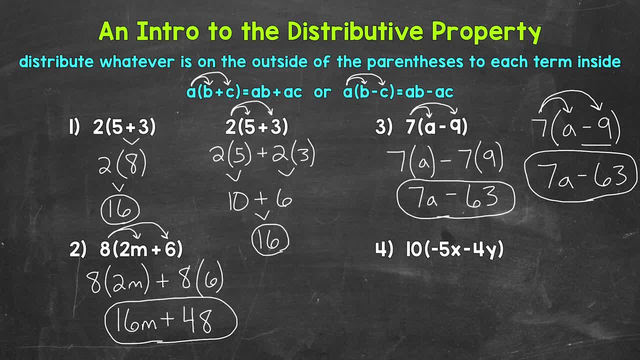 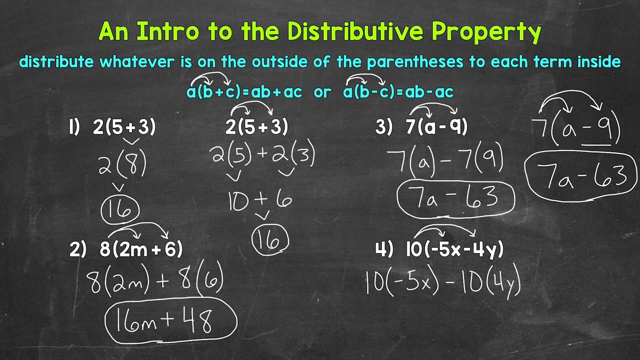 negative five x minus four y. Let's distribute the 10 to the negative five x and to the four y, So 10 times negative five x minus 10 times four y. 10 times negative five x gives us negative 50 x minus 10. 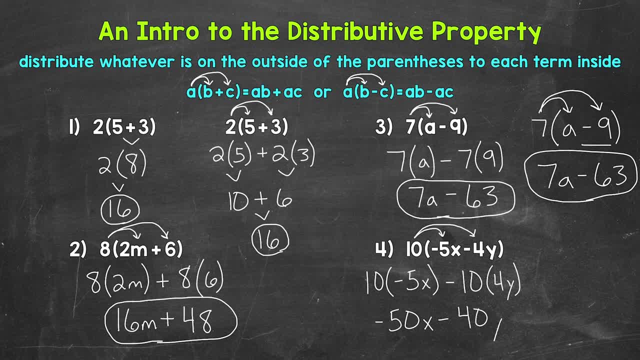 times four y gives us 40 y, So we end up with negative 50 x minus 40 y. We don't have any like terms that we can combine, So we are done Again: negative 50 x minus 40 y. Now let's take a look at a different way to think. 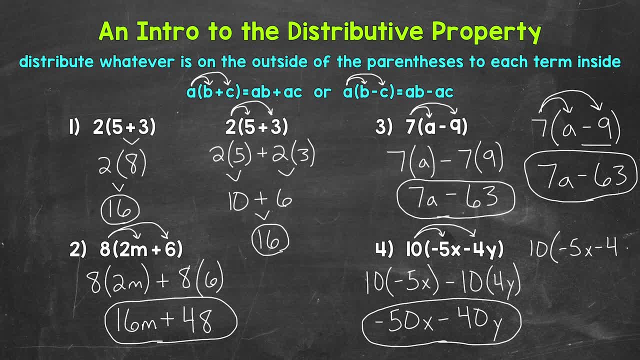 through this, So I will rewrite the expression off to the side. So let's distribute the 10 to the negative five x, And then we will think of that as negative four y. So include the sign in front of that term: 10 times negative five x minus 40 y. So we have a negative five x minus 40 y, And then we 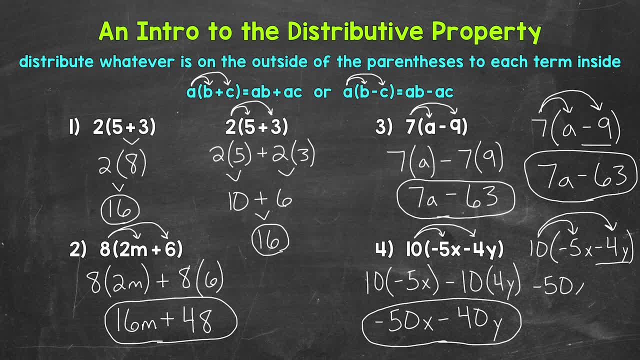 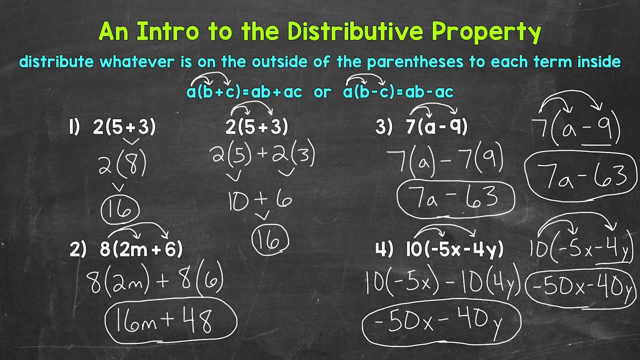 get the same thing that way as well. Negative 50 x minus 40 y. So there is an introduction to the distributive property. Let's take a look at four more examples. Here are more examples that we can go through to get the distributive property. So let's take a look at four more examples. 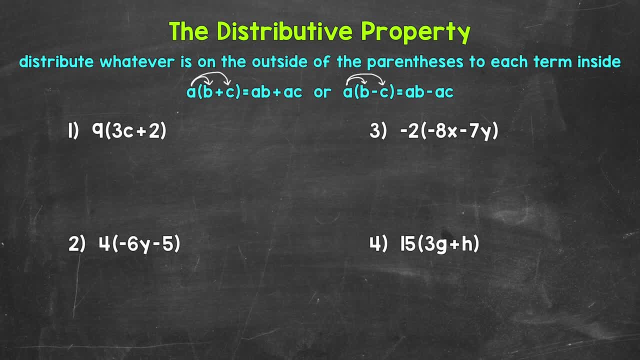 Let's jump into number one, where we have nine and then three c plus two in the parentheses. Let's distribute that nine to the three c and to the two, So we have nine times three c, which is 27 c plus. So we bring that addition sign down And then we have nine times two, which is 18.. So we end. 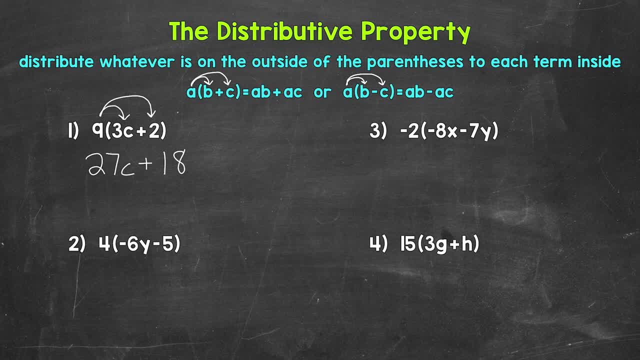 up with 18.. Now we don't have any like terms that we can combine, So this has been simplified. We can't simplify any further. So again: 27 c plus 18.. Let's move on to number two, where we have four and 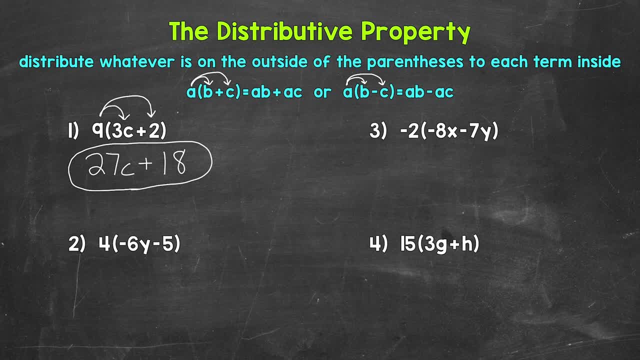 then in parentheses, negative six y minus five. Let's distribute that four to the negative six y and to the five, So four times negative six y, So we end up with negative 24 y minus 20.. We don't have any like terms that we can combine, So this is: 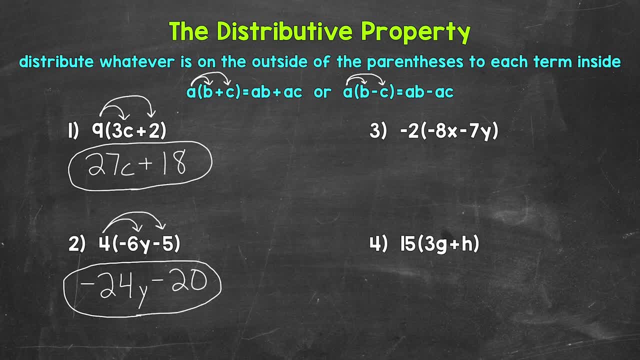 simplified Again: negative 24 y minus 20.. Now I do want to mention another way to think through number two, And this is an option when we have subtraction. So we have negative 24 y minus 20.. So let me rewrite the expression here. 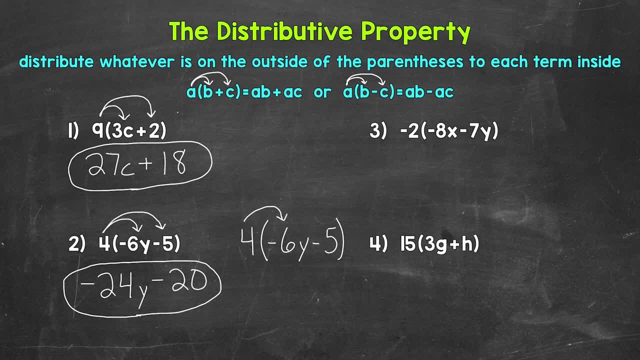 And then we need to distribute the four. So distribute to the negative six y, And then when we distribute to the five, we are going to look at this as negative five. So we are including that subtraction sign, The sign in front of the five, And look at this as negative five. This gives us: 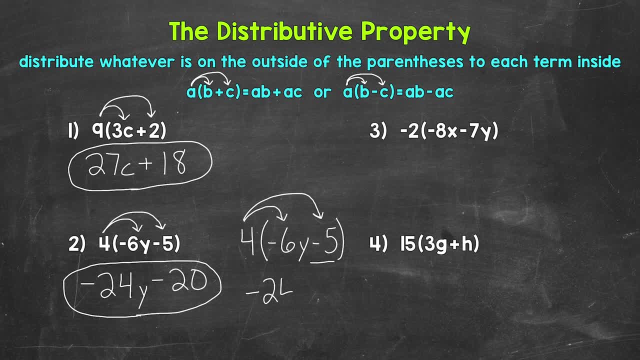 well, four times negative six y minus 20.. So we have negative 24 y minus 20.. And then we need to distribute the four, So we have negative six y minus 20.. So we have negative 24 y minus 20.. And then 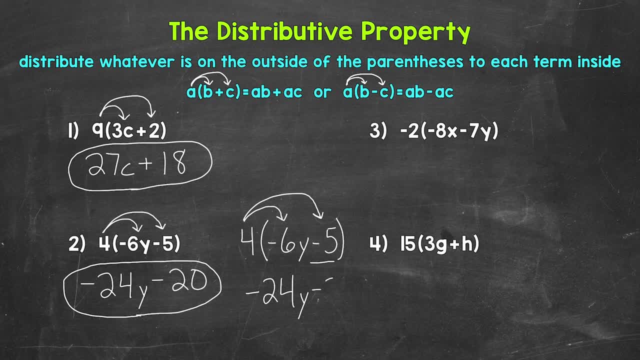 four times negative. five is negative 20.. So we get negative 24 y minus 20.. That way as well. So we get the same thing either way, just slightly different. as far as working through the distributive property, Let's move on to number three, where we have negative two and then in. 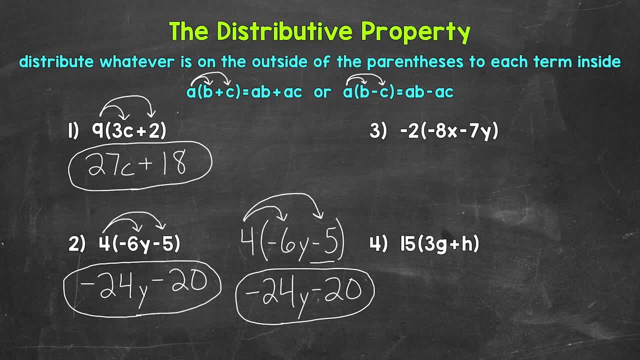 parentheses: negative eight x minus seven y. Let's distribute that four to the negative: six y minus 20.. the negative two to the negative eight x and to seven y, So negative two times. negative eight x gives us 16 x. Remember a negative times. a negative is a positive, So negative two times. 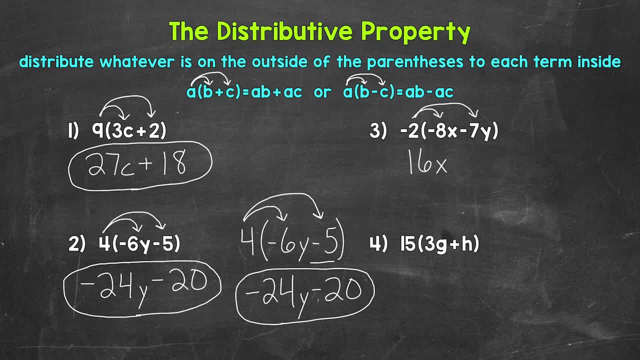 negative eight is a positive 16. And then we have that x, Then we can bring down the subtraction sign, And then we have negative two times seven y. That gives us negative 14 y. Now, this is correct, But we can clean this up a little bit. so to speak, We have: 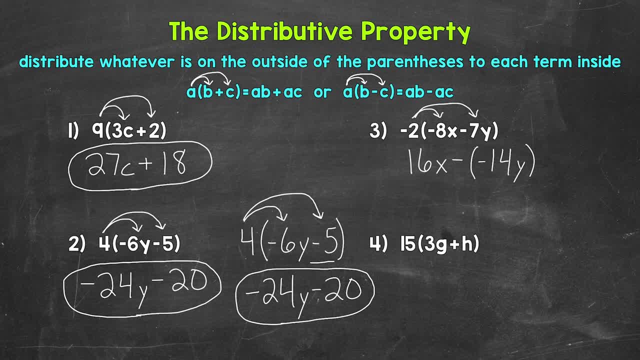 a double sign: The subtraction and then the negative. We don't need both of those signs. We can rewrite it with just one. Think about working with negatives. When we subtract a negative, that's the same as adding a positive. We can change this to addition and that will make 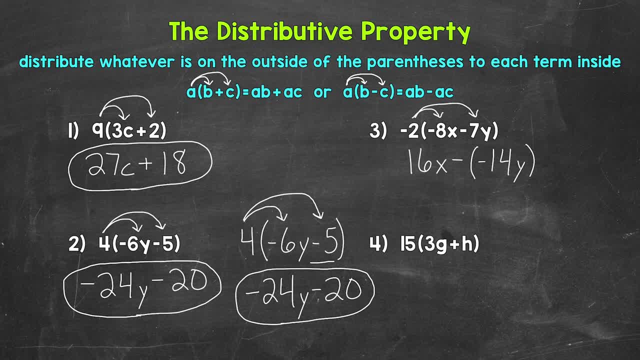 this simpler And, like I said, clean it up a little bit. We can rewrite this as 16 x plus 14 y. We don't have any like terms that we can combine, So we are simplified again: 16 x plus 14 y. 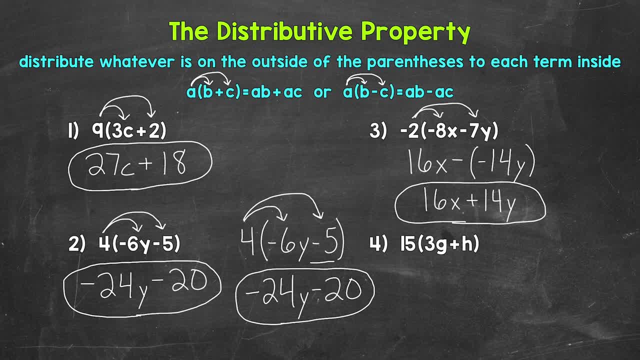 Just like number two. I'll go through this a slightly different way as far as thinking through the distributive property. when it comes to subtraction, I will rewrite the expression off to the side here, And then we can distribute that negative two to the negative eight x, And then we can distribute. 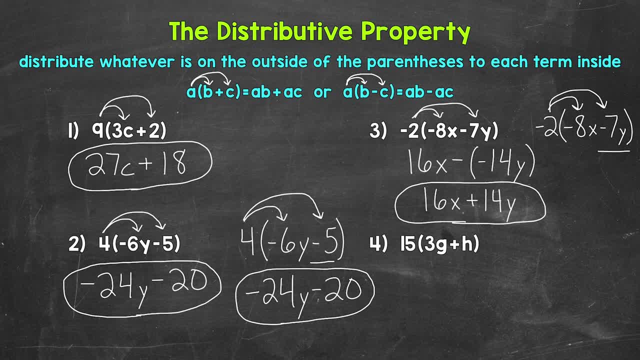 that negative two to the negative seven y. So we are including that sign in front of the term. Negative two times negative eight x gives us 16 x. Negative two times negative seven y gives us a positive 14 y. So plus 14 y, So we get the same. 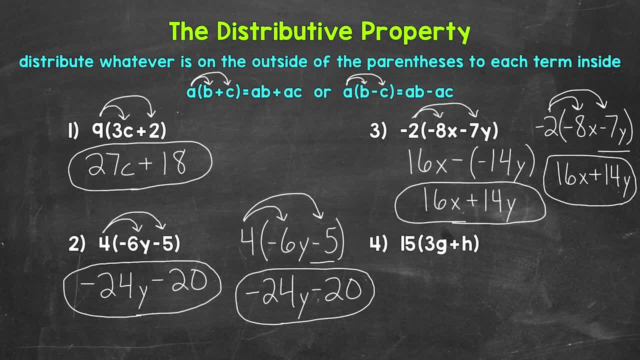 thing there as well. Lastly, let's move on to number four, where we have 15 and then 3g plus h in the parentheses. So let's distribute that 15 to the 3g and to the h, So we have 15 times 3g. 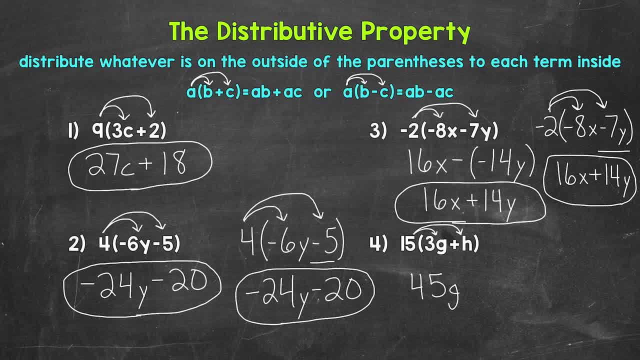 That gives us 45 g plus, and then 15 times h, Well, that's just 15 h, So we end up with 45 g plus 15 h. We don't have any like terms that we can combine, So we can't simplify this any further. 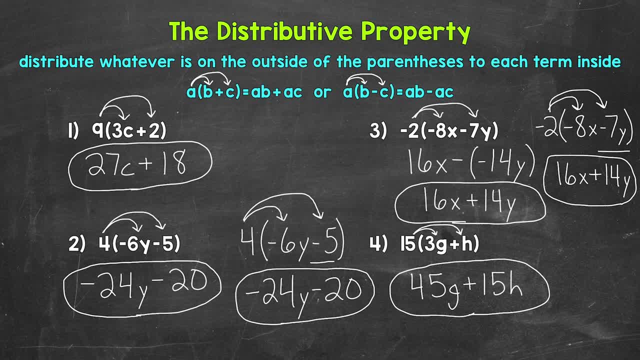 This is simplified. So again, 45 g plus 15 h. So there are the basics of using the distributive property to simplify. So let's go ahead and do that, So let's go ahead and do that, So let's go ahead, and. 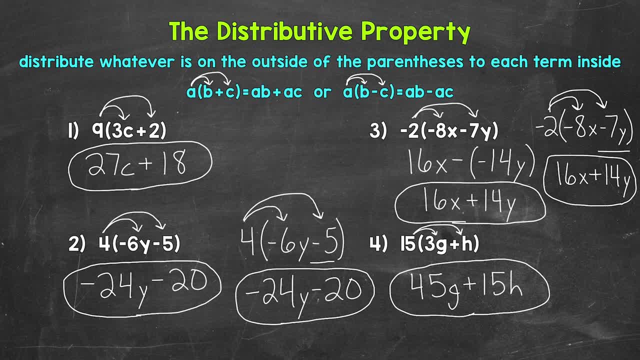 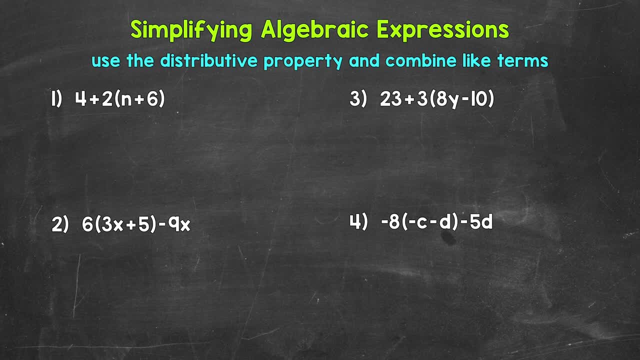 more algebraic expressions that we need to simplify. We will use both the distributive property and combining like terms. Let's jump into number one, where we have 4 plus 2 and then, in parentheses, n plus 6.. So let's go ahead and do that. So let's go ahead and do that. So let's. 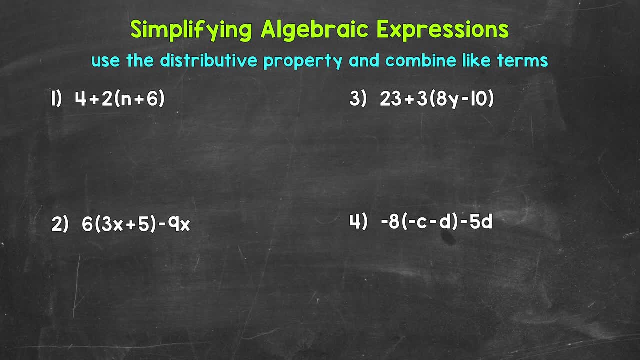 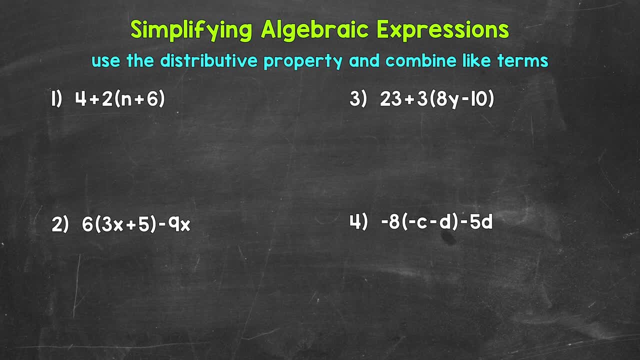 are unlike terms, So we can't combine those terms. What we can do is use the distributive property to remove the parentheses and then we can look to combine like terms to simplify the expression further. So let's distribute the 2 to the n and to the 6.. 2 times n gives us 2n, and then 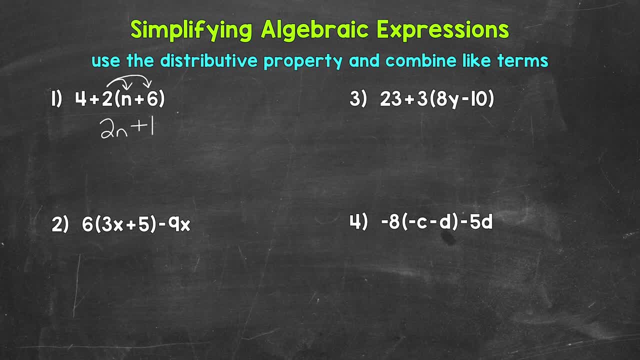 we have 2 times 6, which gives us a positive 12. so plus 12.. This is a positive 2n and then we can bring down that 4.. Now that the parentheses have been removed, we can look to simplify further by combining like terms. 4 and 12 are like terms. Those are constant terms, so we can combine them. 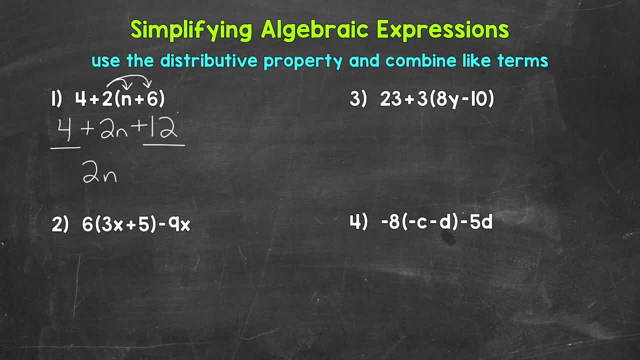 4 plus 12 gives us 16. so our final simplified expression is 2n plus 16.. Now when we write expressions, typically speaking, we want any variable terms first and then constant terms go last. so that's why we have 2n plus 16.. 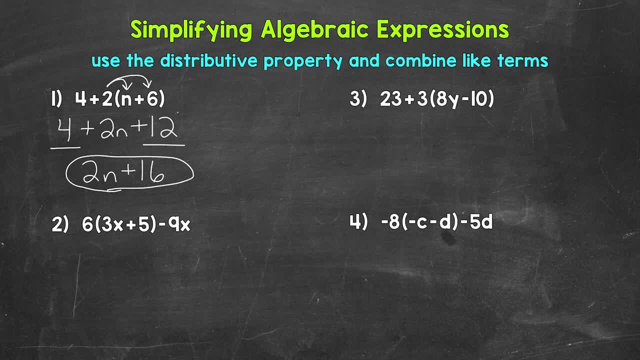 If we end up having multiple terms that involve variables, they go in order from greatest to least as far as exponents, and then, if variable terms have the same exponents go in abc order. So again for number one, we just have two terms: a variable term and then a constant term. so 2n plus 16 is 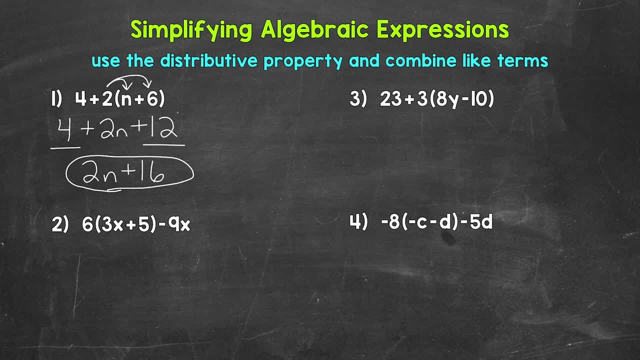 our final simplified expression. Now that final simplified expression is equivalent to the original expression. We were just able to simplify that original expression by using the distributive property and combining like terms. Let's move on to number two, where we have 6 and then in parentheses 3x plus 5 and parentheses minus 9x. Let's start by using the distributive. 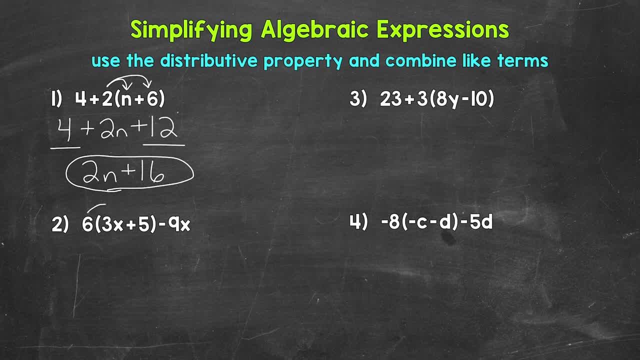 property. to remove the parentheses. So let's distribute this: 6 to the 3x, to the 5. 6 times 3x gives us 18x, and then 6 times 5 gives us a positive 30, so plus 30. Then we 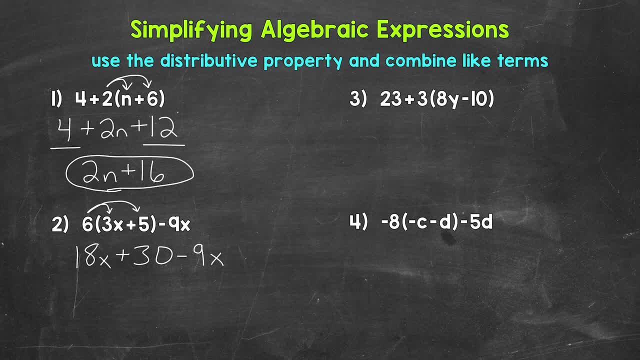 have minus 9x, so a negative 9x. Now that we removed the parentheses, we can look to combine like terms. 18x and negative 9x are like terms, so we can combine them To include the sign that's in front of a term that's negative 9x. So we have 18x minus 9x, or. 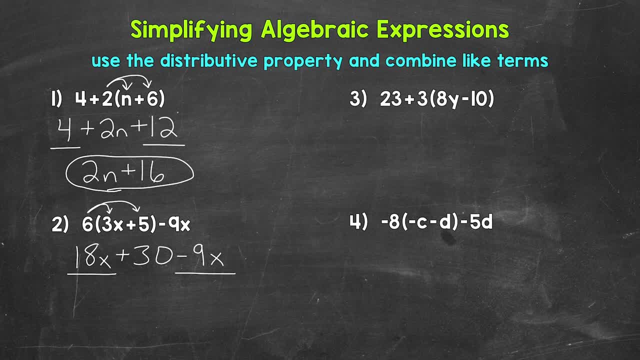 18x combined with negative 9x, That gives us a positive 9x, and then we have plus 30, a positive 30. So our final simplified expression is 9x plus 30. Let's move on to number three, where we have: 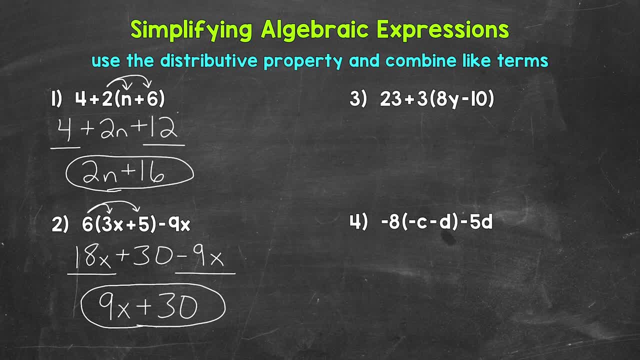 plus 3 and then in parentheses, 8y minus 10.. Let's remove the parentheses by using the distributive property. So let's distribute the 3 to the 8y and to the negative 10.. 3 times 8y. 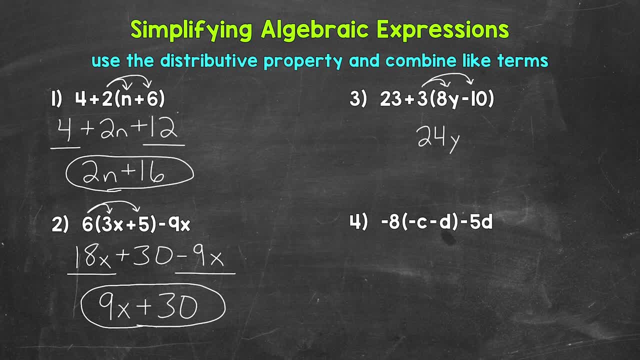 gives us 24y, and then 3 times negative 10 gives us negative 30. This is a positive 24y, and then we have minus 9x plus 3 and then in parentheses, 8y minus 10.. Let's remove the parentheses. 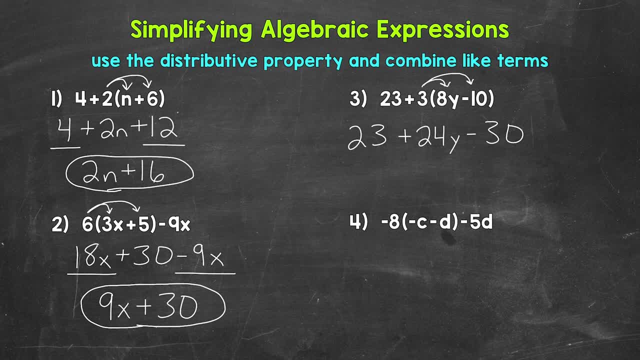 and bring down the 23.. Now, as far as the distributive property and subtraction, we can also think through that as 3 distributed to 8y. So 3 times 8y, that gives us 24y. Then we can bring the subtraction sign down and then distribute the 3 to the 10. So 3 times 10, that gives us 30. So 24y. 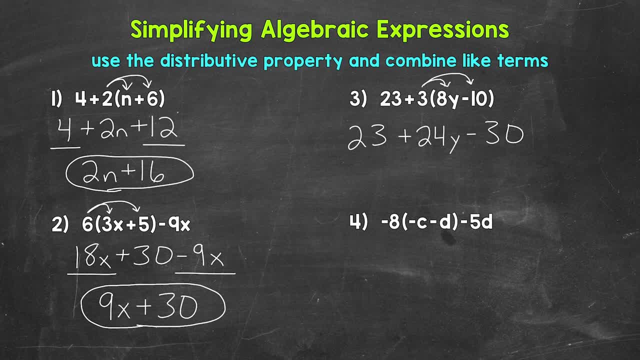 minus 30. We got the same thing thinking through the distributive property that way as well. Now that we removed the parentheses we can look to combine like terms. We have two constant terms, 23 and negative 30. So we can combine those like. 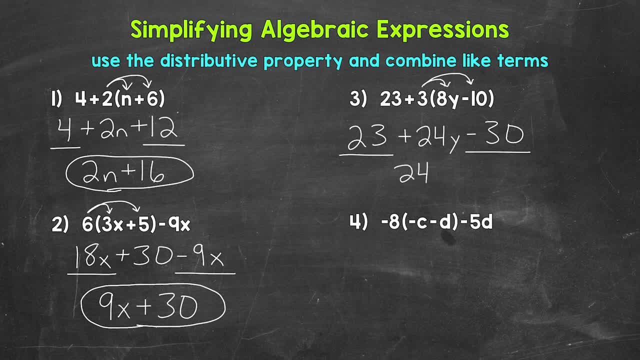 terms. So we have 24y, and then 23 minus 30, or 23 combined with negative 30 gives us negative 7.. So minus 7.. Simplified expression: 24y minus 7.. Lastly, let's move on to number 4, where we have negative 8 and 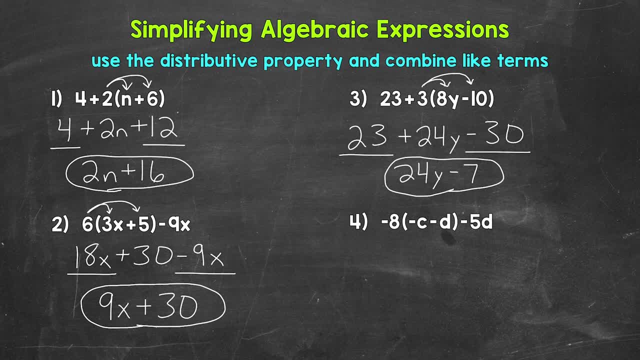 then in parentheses negative c minus d and parentheses minus 5d. Let's start by removing the parentheses by using the distributive property. Distribute the negative 8 to the negative c and distribute the negative 8 to negative 8.. d- Negative 8 times negative c gives us a positive 8c. Remember a negative times a negative equals. 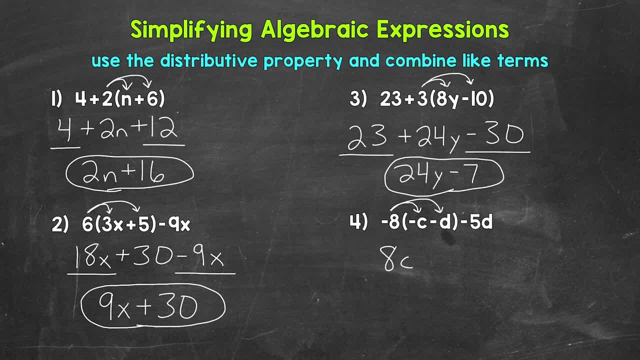 a positive Negative 8 times negative. d gives us a positive 8d And then we have minus 5d, so a negative 5d. Now that we removed the parentheses we can look to combine like terms. 8d and negative 5d are like terms, So let's combine those like terms. We end up with 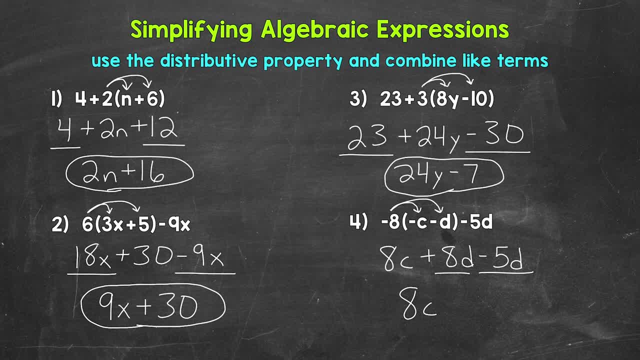 8c, and then 8d minus 5d, or 8d combined with negative 5d gives us a positive 3d, So plus 3d. Our final simplified expression: 8c plus 3d. So there's how to use the distributive property. 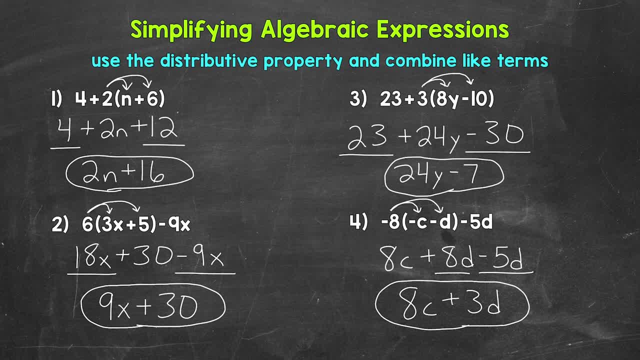 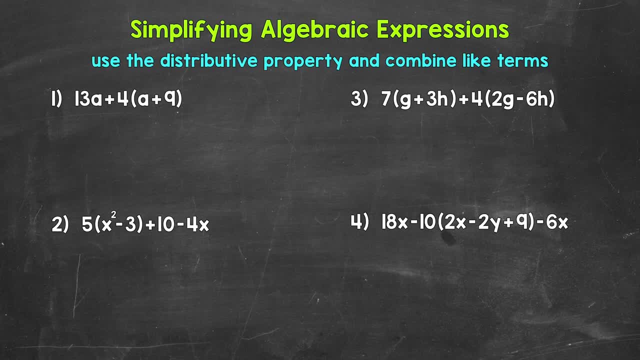 and the derivative property, Combining like terms to simplify an algebraic expression. Let's take a look at four more examples, and these will get a little more complex. Here are four more algebraic expressions that we need to simplify using the distributive property and combining like terms. These will get a little. 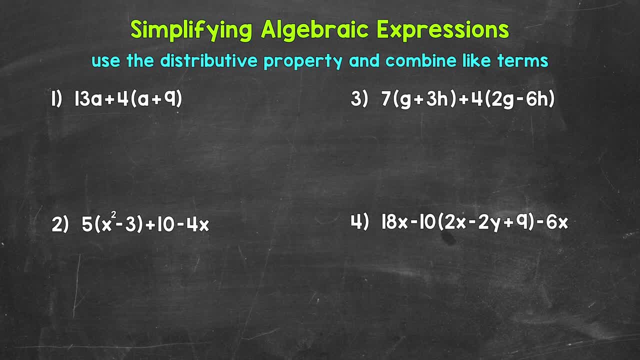 more complex than the previous four examples. Let's jump into number one, where we have 13a plus 4 and then in parentheses, 9.. Now, since we have parentheses, we need to start there. We can't combine the terms in the. 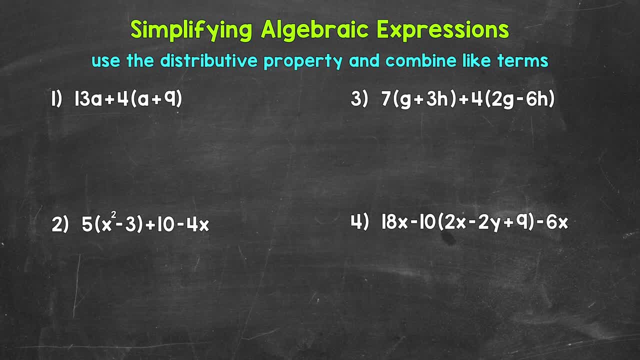 parentheses. They are unlike terms, So we can use the distributive property to remove the parentheses. Once the parentheses are removed we can look to combine like terms. So let's distribute that 4 to the a and to the 9. So we have 4 times a, which is 4a, And then we can look. 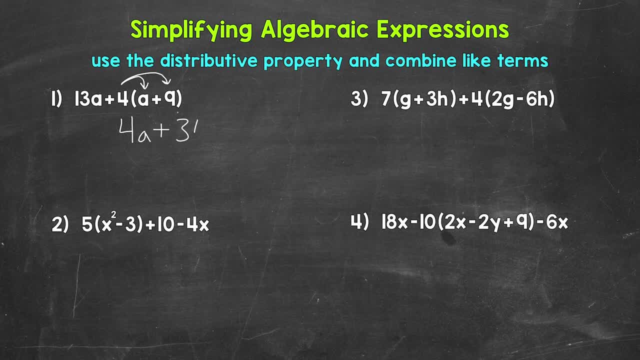 at 4 times 9.. And then 4 times 9 is a positive 36.. So plus 36.. This is a positive 4a, And then we can bring down 13a. Now that we removed the parentheses, we can look to combine like terms in order to: 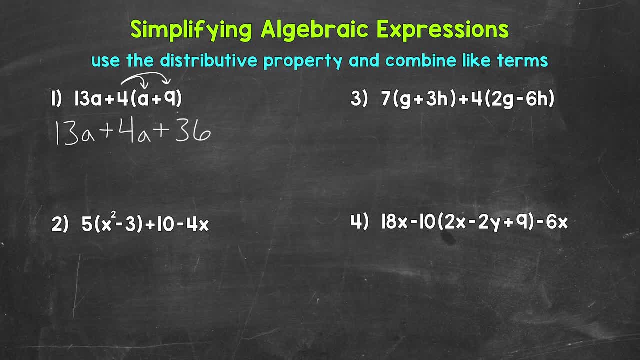 simplify this further. So do we have any like terms that we can combine? Yes, 13a and 4a are like terms, So we can combine those terms And then we can bring down 13a, And then we can bring down 13a, And then we can. 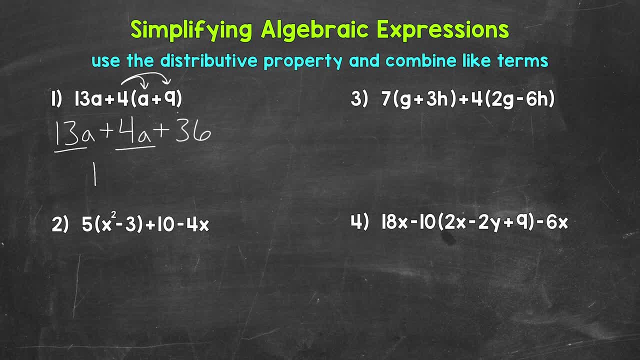 bring down those terms: 13a plus 4a is 17a, And then we have that positive 36.. So plus 36.. And this is our final simplified expression: 17a plus 36.. Now that simplified expression is equivalent. 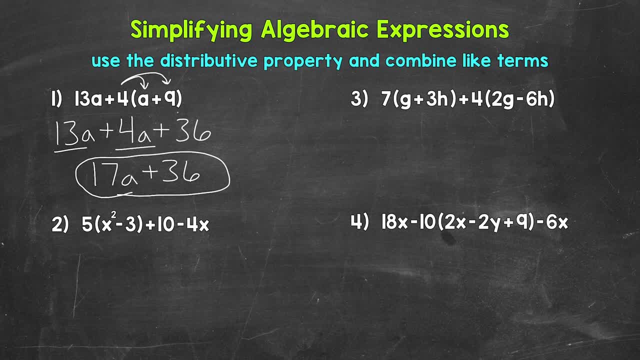 to the original expression. We were just able to simplify that original expression by using the distributive property, And then we can look to combine those terms. So we can look to combine like terms. Let's move on to number 2, where we have 5.. And then, in parentheses, x squared minus. 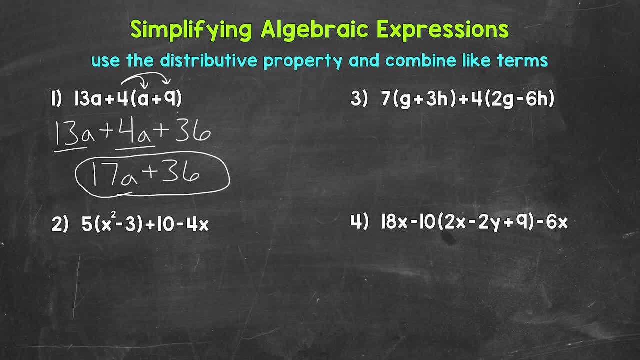 3. End parentheses. Plus 10, minus 4x. Let's start by using the distributive property in order to remove the parentheses. Then we can look to combine like terms. Let's distribute this 5 to the x squared and to the negative 3. 5 times x squared. 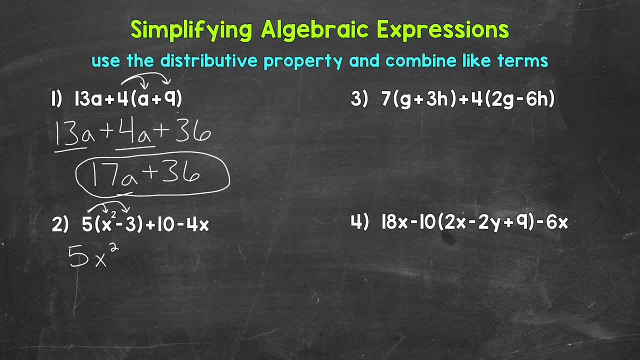 Gives us 5x squared, And then 5 times negative 3 gives us negative 15.. Now another way to think through that distributive property there is to do 5 times x squared, which is 5x squared, Bring the subtraction sign down and then do 5 times 3.. We get 5x squared minus 15. that way, as 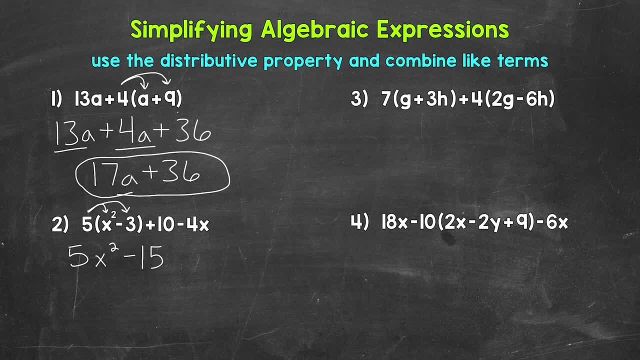 well, Just a slightly different way to think through the distributive property. Then we have positive 10.. So plus 10.. And then a negative 4x, So minus 4x. Now that we removed the parentheses, we can look to combine like terms. So do we have any like terms that we can combine? Yes, 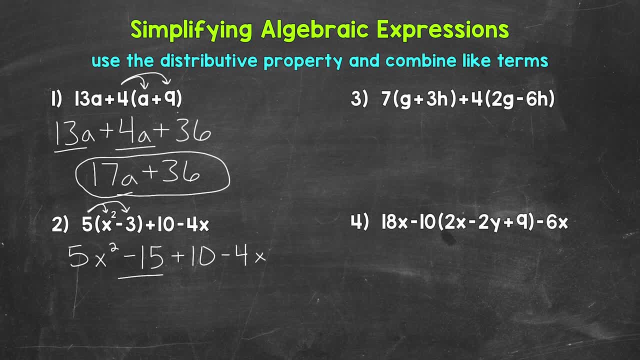 we have two constant terms, negative, 15 and 10.. So let's combine those like terms. So we have 5x squared minus 15. And then we have 5x squared minus 15. And then we have 5x squared minus 15.. And then we have: 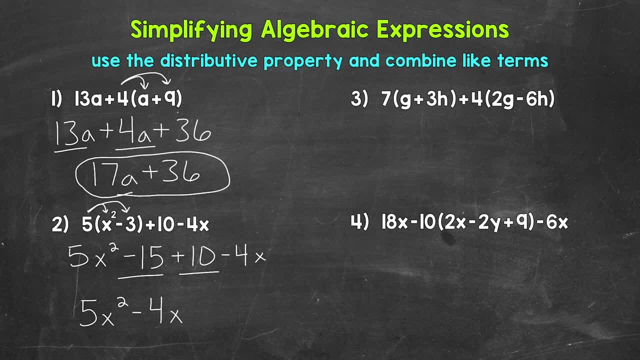 negative 4x. That's a negative 4x. The term will take the sign that's in front of it. So make sure we have negative 4x there, And then the constant term comes last, So we have negative 15 plus 10 or 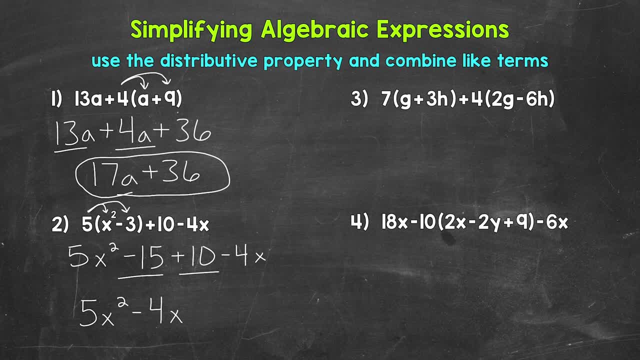 negative 15 combined with positive 10. That gives us negative 5.. So minus 5.. And this is our final simplified expression: 5x squared minus 15.. And then we have negative 4x squared minus 15.. And then 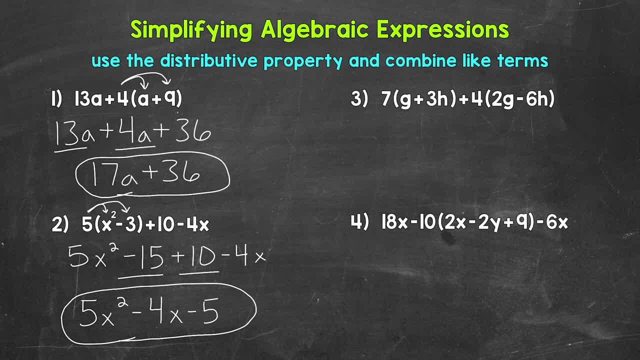 we have negative 4x squared minus 15.. And then we have negative 4x squared minus 15.. And then we have Now. I do want to mention as far as how this simplified expression is written. Typically speaking, when writing expressions, the greatest exponent comes first, So greatest to least If 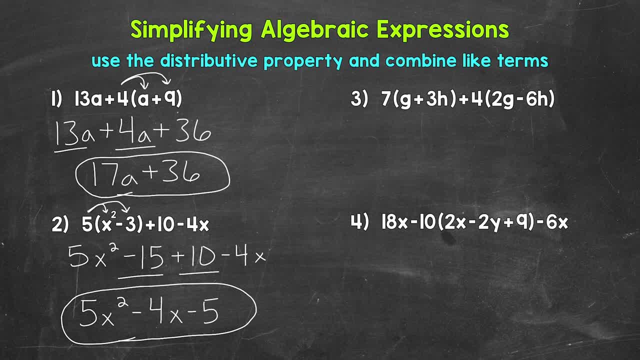 exponents are the same, go in ABC order. Constant terms go last. So we have 5x squared. The exponent of 2 comes first because that's the greatest exponent. Then we have negative 4x, So that variable has an understood exponent of 1.. Remember, whenever there isn't an exponent, 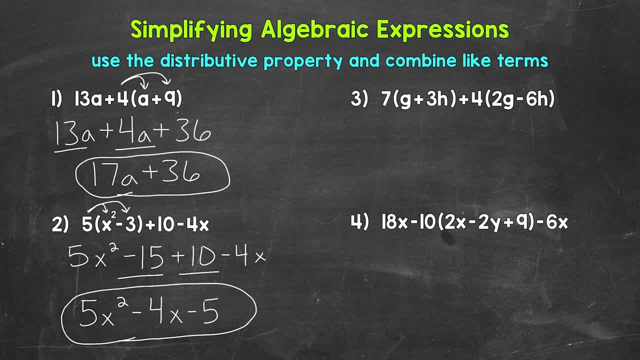 written, there is an understood exponent of 1,, so to the power of 1.. Anything to the power of 1 is just itself. And then we have the constant term of negative 5 last. So that's something to keep in mind as far as writing out expressions. Let's move on to number 3, where we have 7, and then 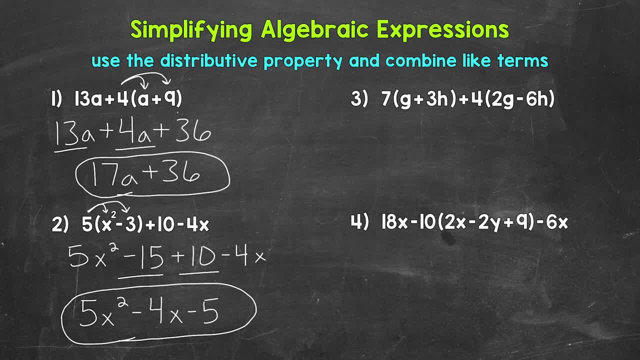 in parentheses g plus 3h and parentheses plus 4, and then in parentheses 2g minus 6h. Let's start by using the distributive property to remove any parentheses and then we can look to combine like terms. Let's distribute this 7 to the g and to the 3h, So we have 7 times g. that gives us 7g. 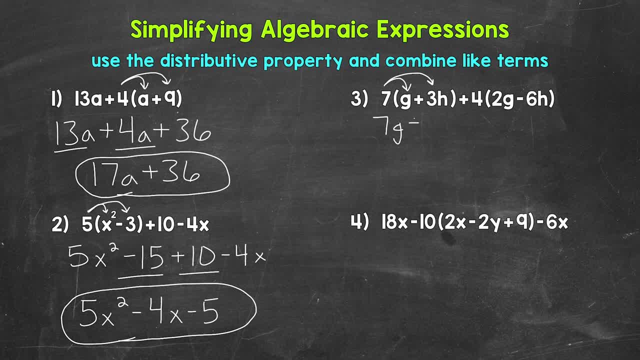 and then we have 7 times 3h. That gives us a positive 21h, so plus 21h. Then we can distribute the 4 to the 2g and to the negative 6h. 4 times 2g gives us a positive 8g, so plus 8g, And then 4 times negative 6h. 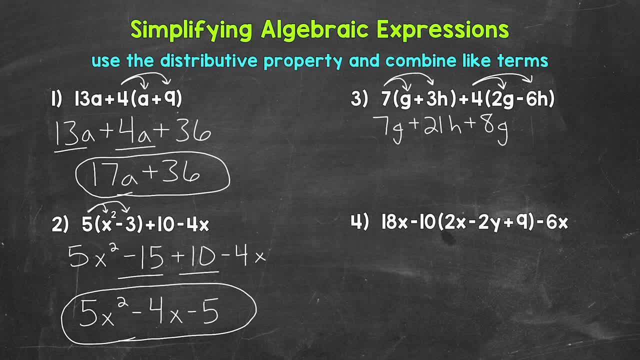 gives us negative 24h A positive times. a negative equals a negative, So negative 24h or minus 24h. Now for this expression. I'm going to rewrite it with all of the like terms next to each other. This is a strategy we can use to organize the expression. 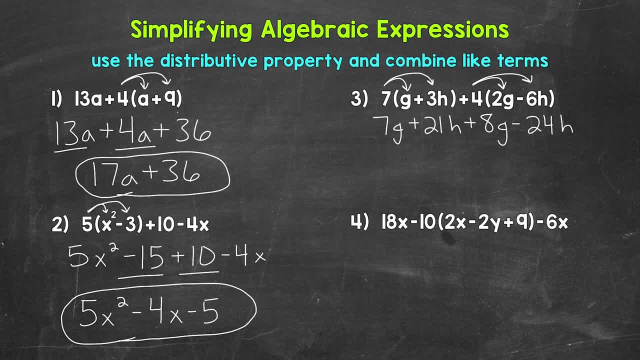 and make combining like terms a little simpler, since all of the like terms will be right next to each other. So let's identify any like terms in this expression. We have 7g and 8g, which I will box in in order to separate, And then negative 24h. Let's rewrite this with those. 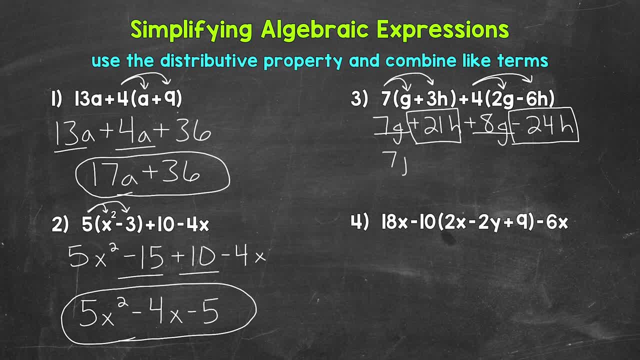 like terms next to each other. So we have 7g plus 8g plus 21h minus 24h. Remember that's a negative 24h. Now all of the like terms are right next to each other, So we have 7g plus 8g plus. 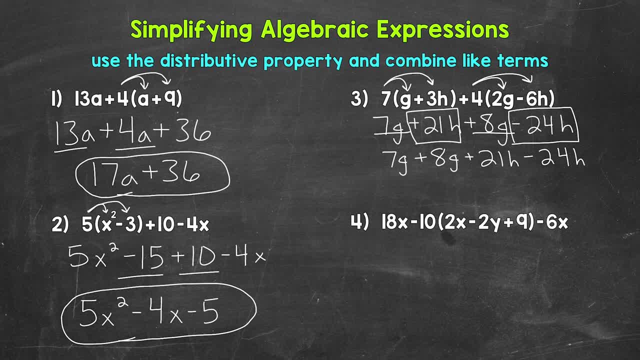 24h. So, like I mentioned, it's a little simpler to combine the like terms. So now we can combine like terms. Let's start with 7g and 8g. 7g plus 8g gives us 15g. Then we have 21h minus 24h. So 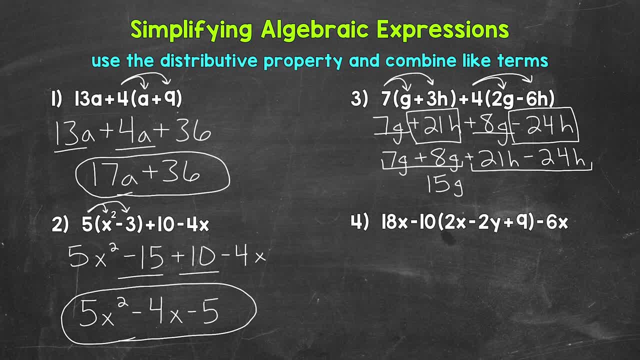 positive 21h. combined with negative 24h, That gives us negative 34h, So minus 3h, And this is our final simplified expression: 15g minus 3h. Lastly, let's move on to number 4, where we have 18x minus 10, and then, in parentheses: 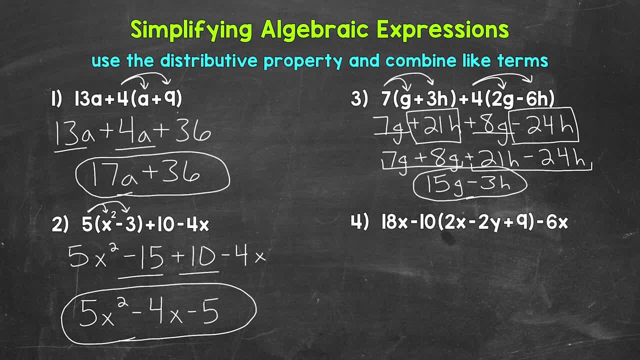 2x minus 2y plus 9, end parentheses minus 6x. Let's start by using the distributive property to remove the parentheses. We're going to distribute negative 10.. We take the sign that's in front, so this is negative 10.. 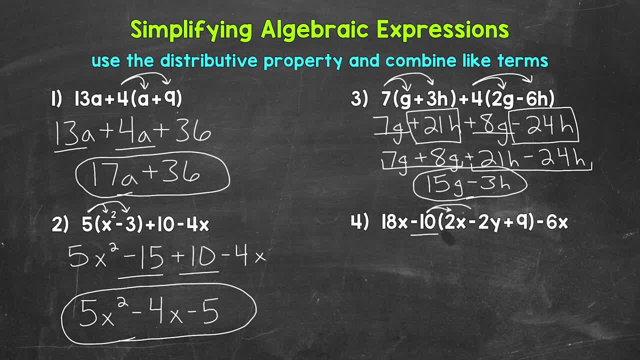 We need to distribute to the 2x, to the negative 2y and to the 9.. Negative 10 times 2x gives us negative 20x. Negative 10 times negative 2y gives us positive 20y. Remember: a negative times a negative equals a positive. And then we have negative 10 times a. 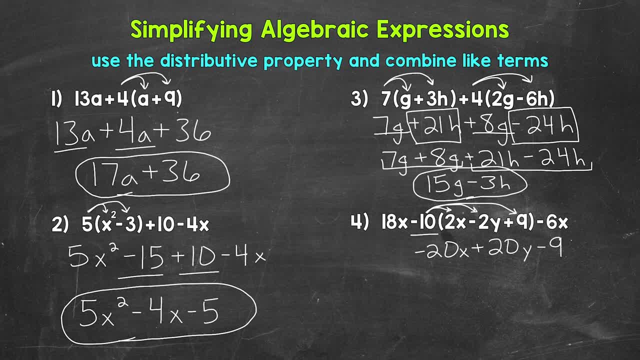 positive 9.. That gives us negative 90. We then have the negative 6x and the positive 18x that we need to bring down. Now we can look for any like terms that we can combine. So do we have any like? 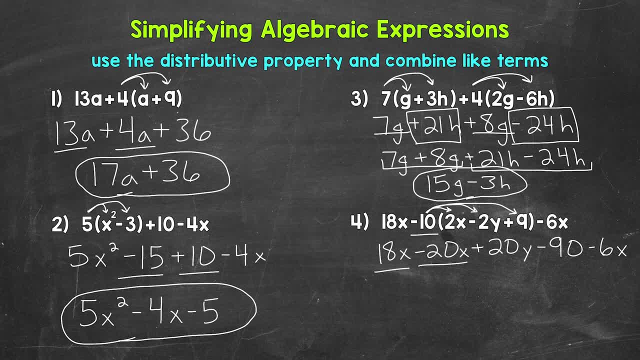 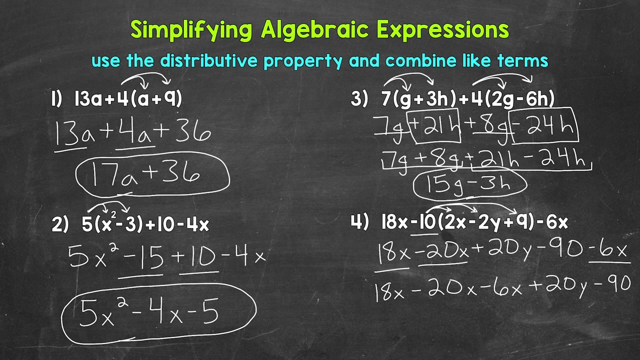 terms: Yes, 18x, negative 20x and negative 6x. Let's rewrite the expression with those like terms next to each other, So 18x minus 20x minus 6x plus 20y minus 90. Now we can combine like terms, So we have 18x. 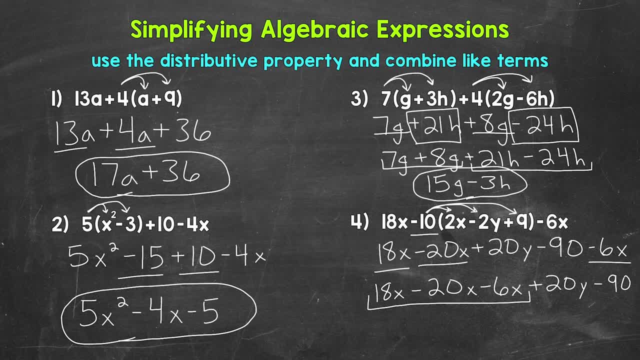 minus 20x, Minus 6x. So we are combining a positive 18x, a negative 20x and a negative 6x. 18x minus 20x is negative, 2x, Negative, 2x minus 6x. that gives us negative 8x. Then we have plus 20y minus 90. So